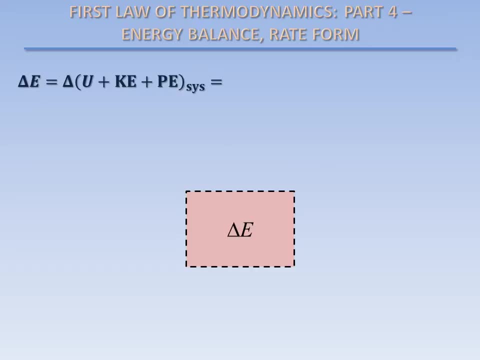 which is equal to the change in the sum of the internal energy, the kinetic energy and the potential energy of the system, is equal to the sum of all of the energy transferred by heat into and out of the system, plus the sum of all of the energy transferred by work into and out. 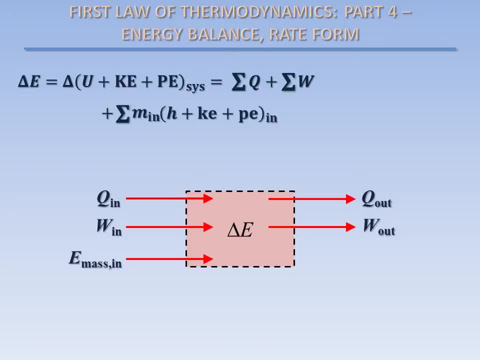 of the system, plus the sum of all of the energy transferred into the system by mass flow, minus the sum of all of the energy transferred out of the system by mass flow. Note that in this energy balance, heat transferred into the system is positive because it increases the total energy. 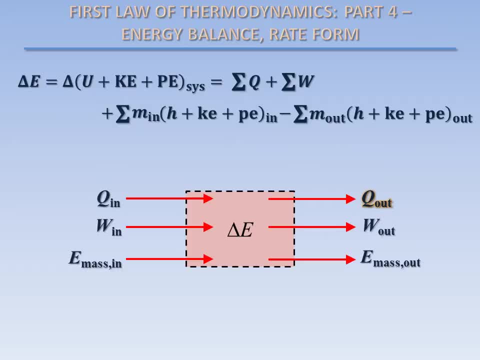 of the system, While heat transferred out of the system is negative because it decreases the total energy of the system. Similarly, work done on the system is positive, while work done by the system is negative. It's useful to write our energy balance in a rate form, especially when mass is flowing. 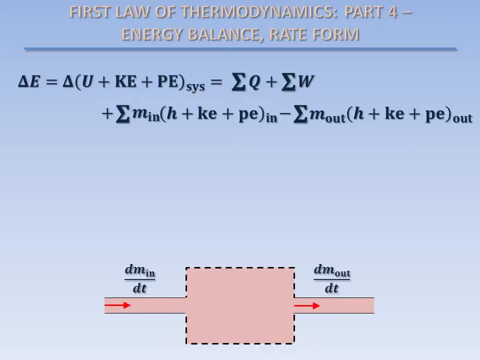 into and or out of our system. The change in total energy of the system with time, or the rate of change of energy of the system, is equal to the sum of all of the energy contained in the system. is equal to the sum of the rate at which heat energy is transferred into and out of the system. 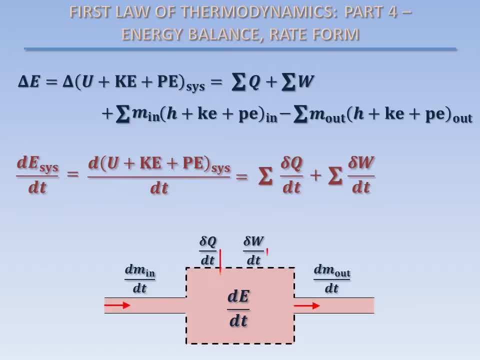 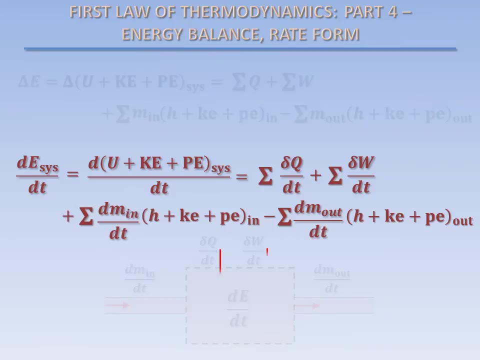 plus the sum of the rate at which work energy is transferred into and out of the system, plus the rate at which energy is transferred into the system by mass flow, minus the rate at which energy is transferred out of the system by mass flow. You may have noticed that there are different symbols used for the time-directed balance. 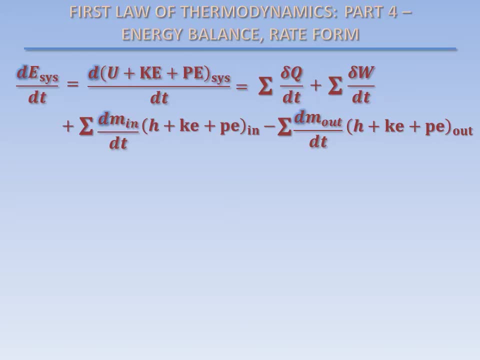 and we're still not at the top of the field of the problem. You could probably tell by the derivatives. Some of these derivatives use the letter D to represent a differential amount. These are called exact differentials. Differential amounts of heat and work are denoted by the delta. 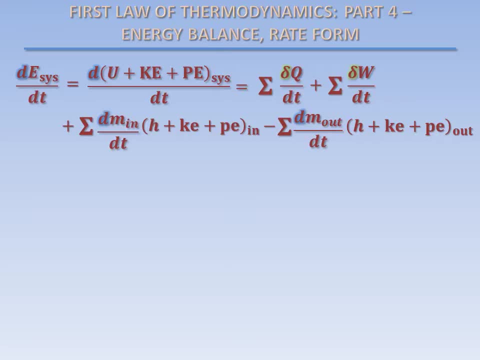 symbol. These are called inexact differentials. Let's take a look at these two types of differentials by comparing the rate of energy change to the rate of heat transfer. Let's integrate the rate of energy change over some process, beginning at time one and ending at time.